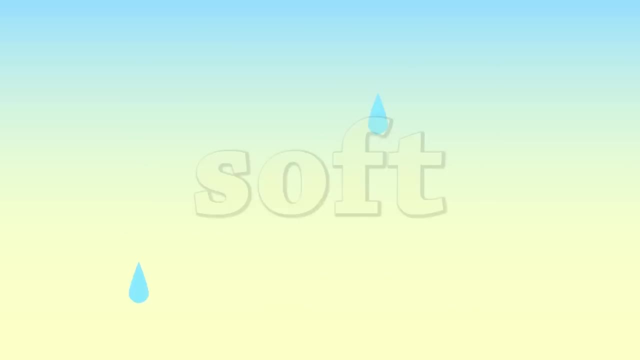 free of salts and therefore soft. However, gases from the air can dissolve in rainwater, and one of these is dissolved carbon dioxide. When rainwater falls on limestone, that's calcium carbonate. the limestone dissolves slowly, which is how the great caves full of stalactites are. 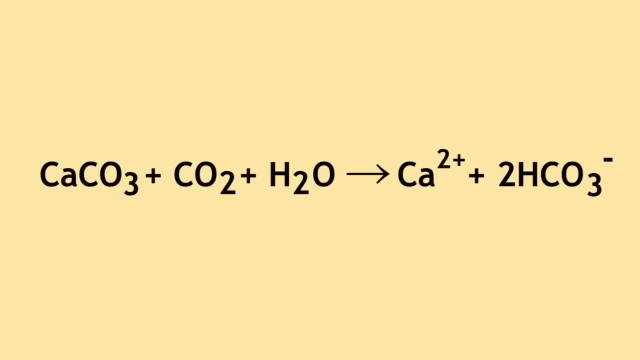 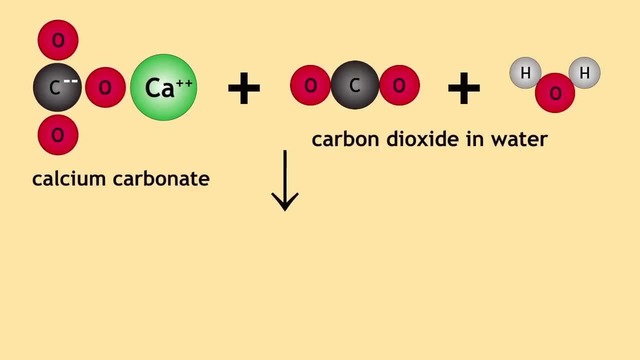 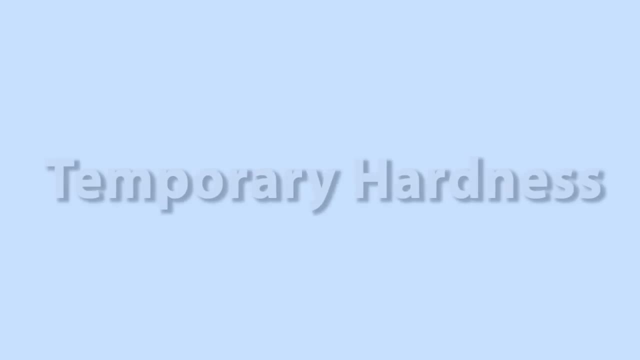 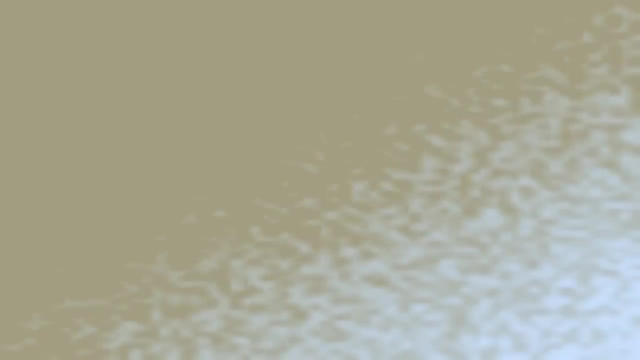 formed. Here's the equation: Calcium carbonate reacts with the carbon dioxide in the rain to form soluble calcium hydrogen carbonate. This form of hardness is called temporary hardness, because boiling reverses the reaction and the hardness is removed, But the limestone will deposit in your pipes, on the cooking utensils or 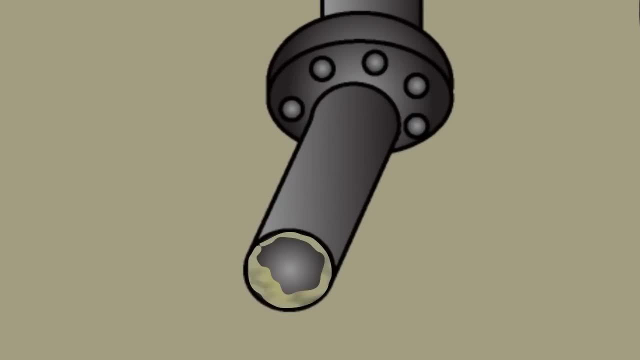 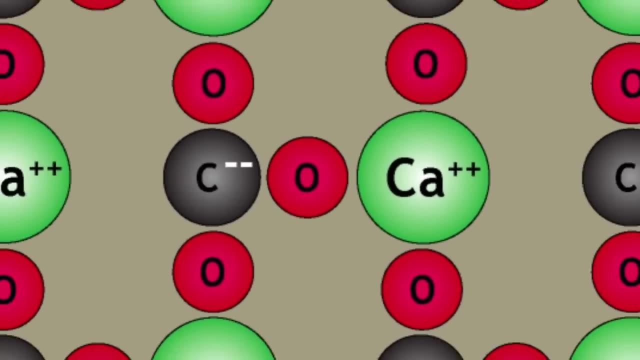 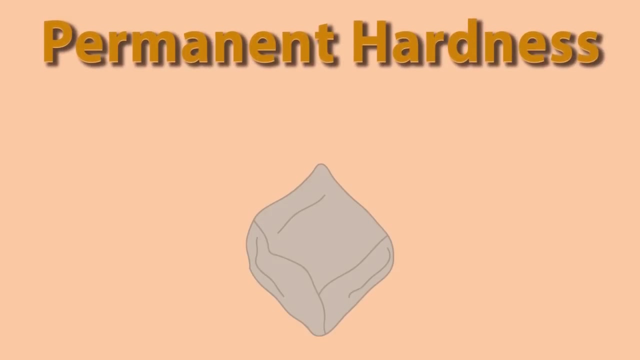 in your kettle, forming something we call lime scale, And this is also how stalactites are formed in those big caves. Another form of hardness is called permanent hardness, which comes from rocks containing gypsum, which is calcium sulphate. In this case, you do not get lime scale. 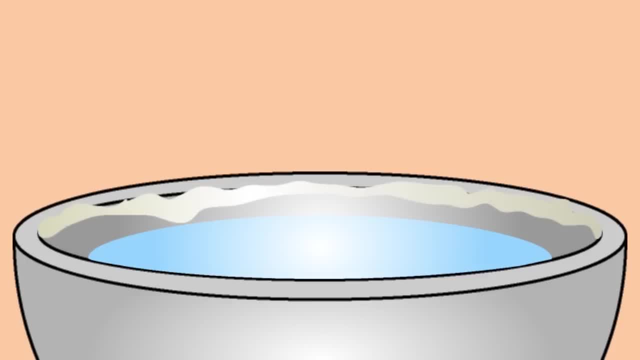 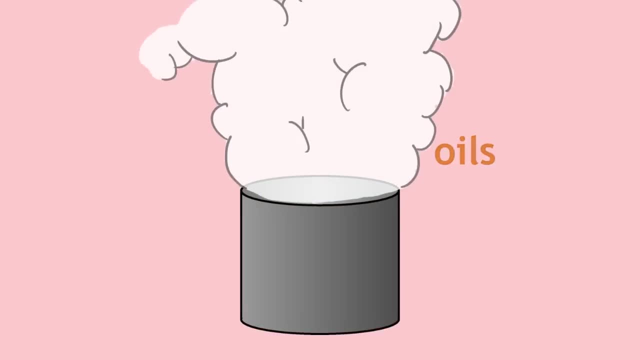 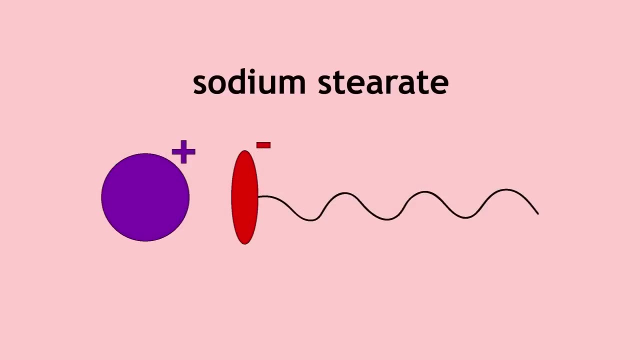 but you still, of course, get a scum with soap. So what is this scum? Well, soap is made by boiling natural fats and oils with sodium hydroxide. The soap molecules, for example sodium stearate, have a long tail, which is attracted to oil or dirt, and the sodium ion end, which is attracted. 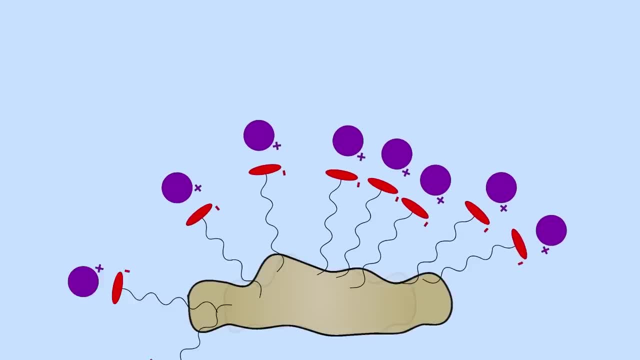 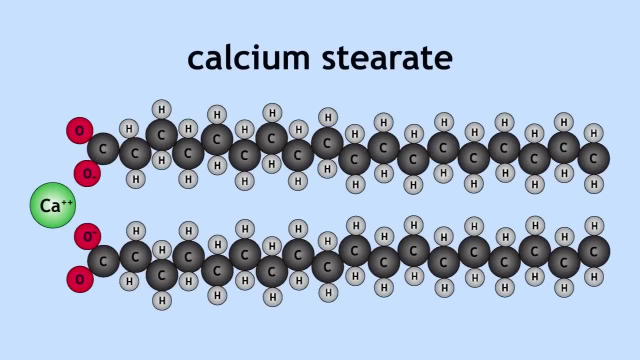 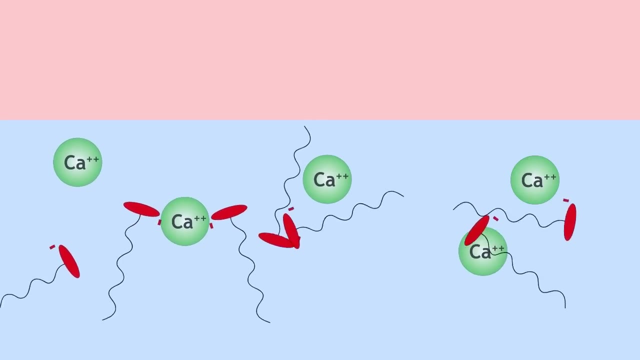 to water. In this way, dirt is lifted off your hand and the clothes and is carried away by the water. However, calcium stearate is insoluble, so if the water contains calcium ions, the soap will not work until all the calcium ions have been precipitated out. as 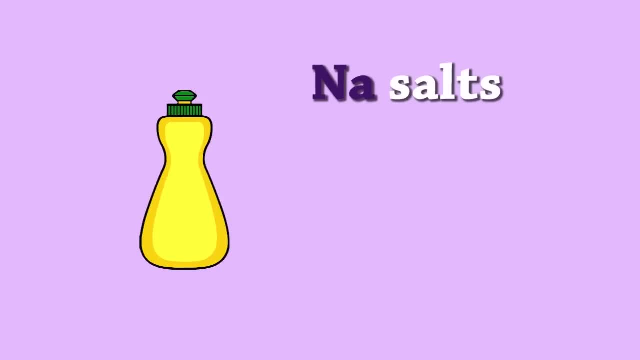 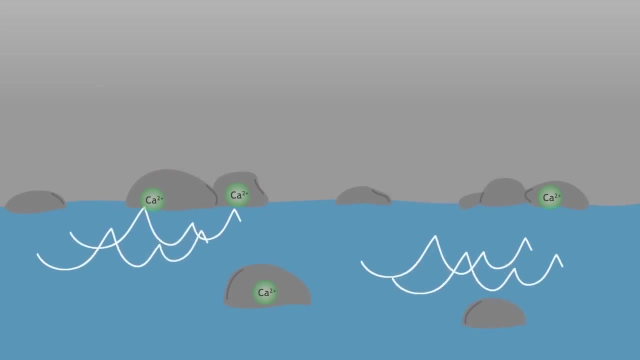 scum. Detergents are sodium salts of compounds called alkyl benzene sulfonates, whose calcium salts are soluble. so there is no problem of scum with detergents. So to summarise, we saw that water becomes hard by flowing through rocks containing calcium.